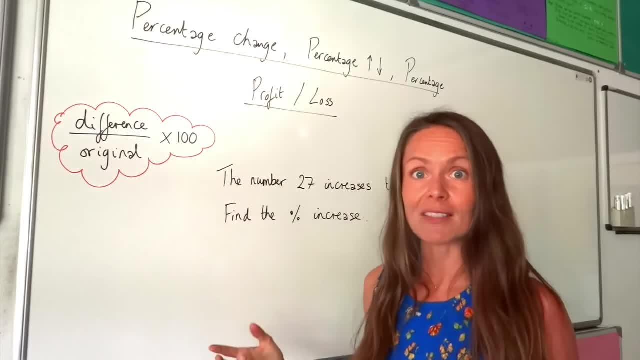 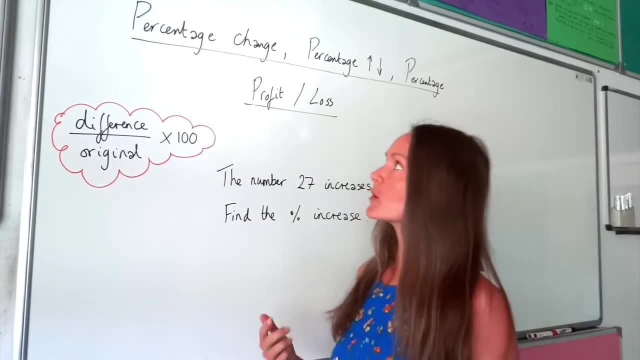 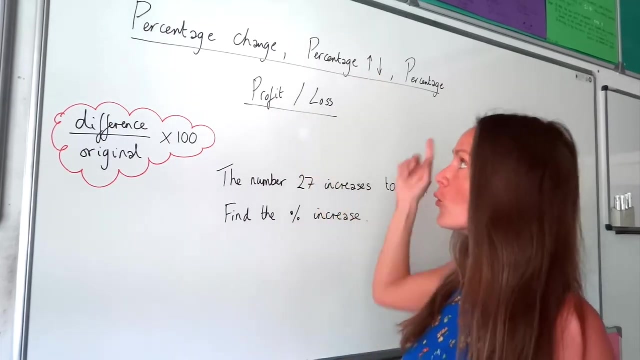 value and then multiply by 100 to turn your answer into a percentage. So this formula works out percentage change. So you can use it for questions talking about percentage increase, percentage decrease, percentage profit and also percentage loss. For all of these questions we use this formula. So in the first question it says the number. 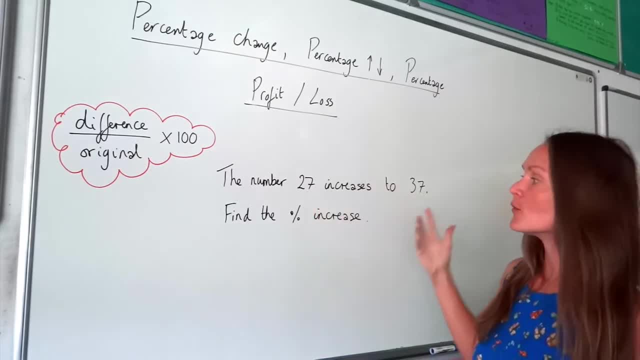 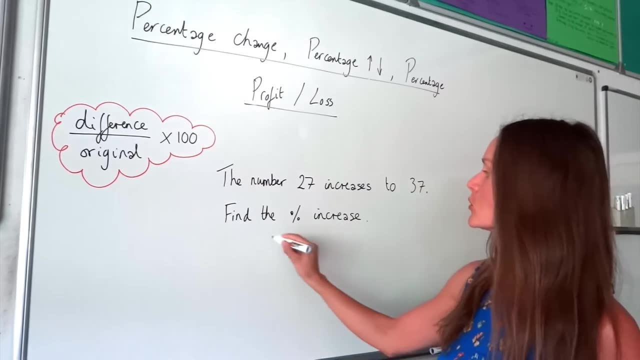 27 increases to the number 37, find the percentage increase. So remember we have to start by finding the difference between these numbers. So you do the larger number 37. Minus the smaller one, because difference means subtract. Then you have to divide by. 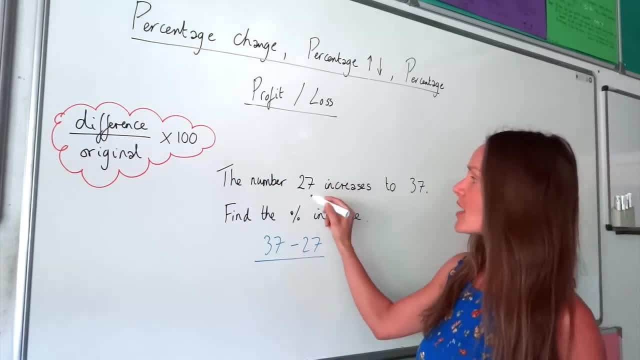 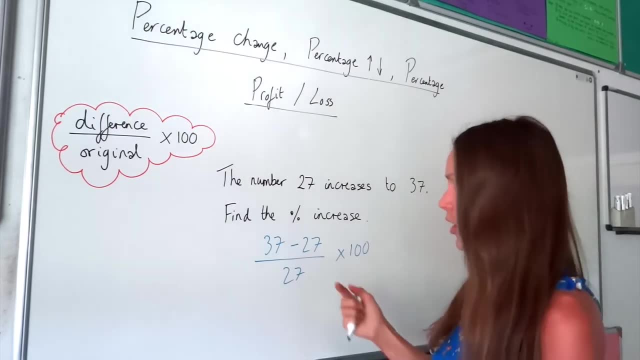 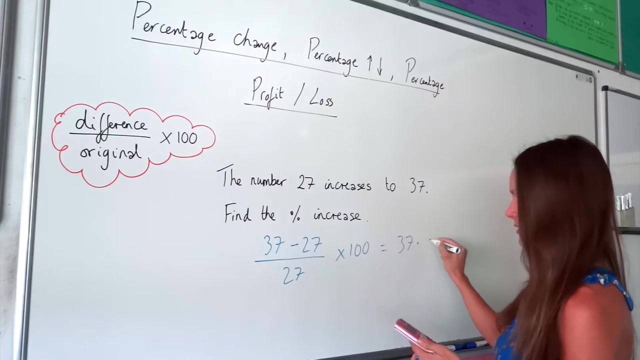 the original value, which is the number it started as, So 27 in this case, Not forgetting to multiply by 100 at the end. So you can pop that in the calculator and we get a decimal answer: It's 37.037, and they're recurring there. So if I round that to three significant 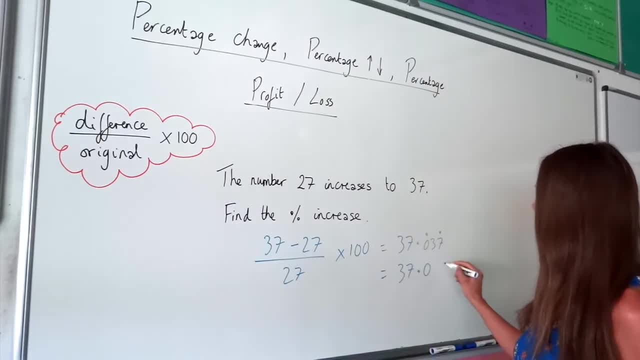 figures, I get 37.037.. So I've got 37.037.. So if I round that to three significant figures, I get 37.037.. Then I add that up, I get 37.037.. Okay, we're going to fill in the. 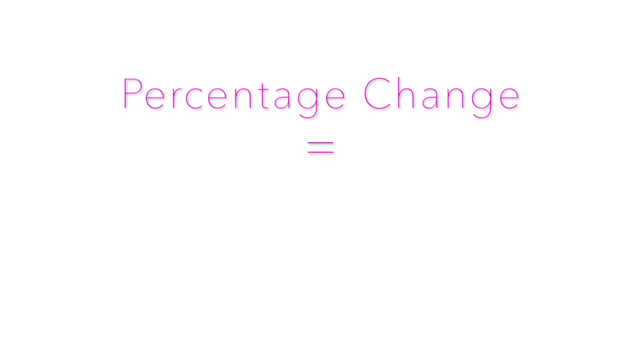 third one, So I get 17.9.. So I'm going to fill it in the third one And if I round that up I get 37.0%. Okay, so there's the first one. Onto the next. Okay. so in this example, I buy a car for 16,350 pounds and I sell it five years later for 11,200.. So, like most cars, it depreciates, It loses value over the first two years. You. 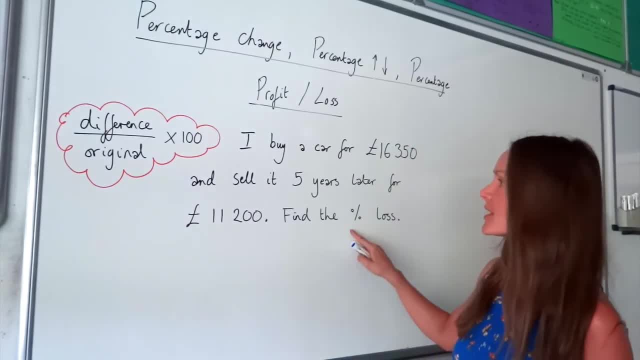 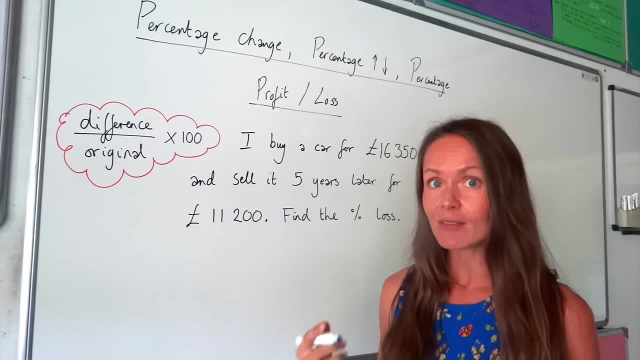 know that's natural time. so we have to work out the percentage loss. so it's exactly the same formula as for the previous question, so this one here. so we have to work out the difference between these two values. so take the larger one, so sixteen thousand. 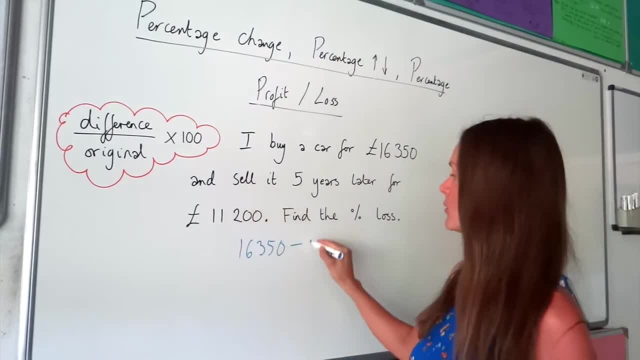 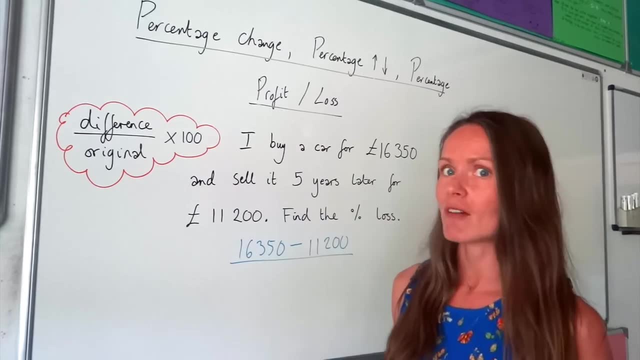 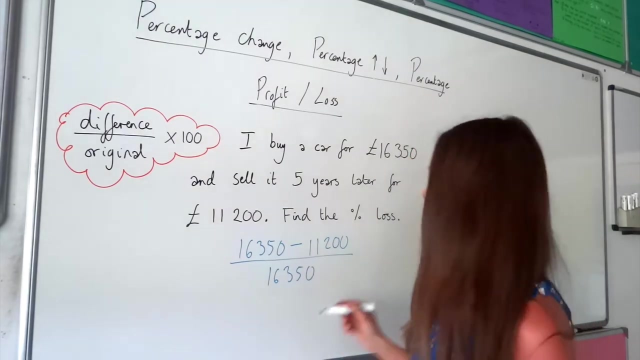 three fifty and minus the smaller value, eleven thousand two hundred, not forgetting to divide by the original value. so that's the value that I bought the car at. so this one here, so sixteen thousand three fifty, and then multiply by one hundred to turn it into a percentage. so pop that in your